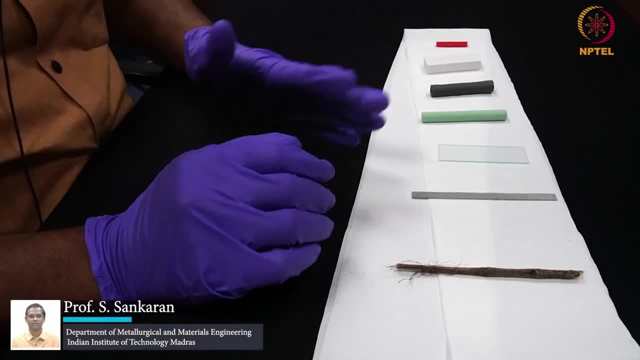 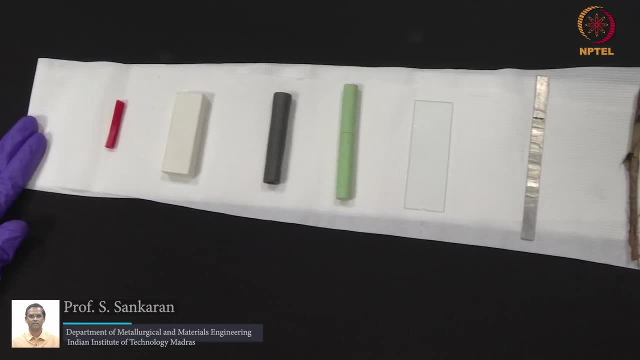 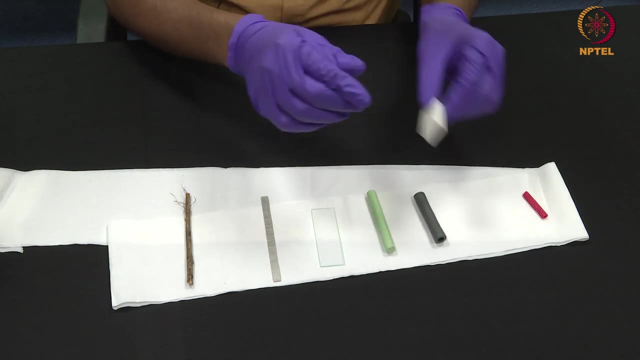 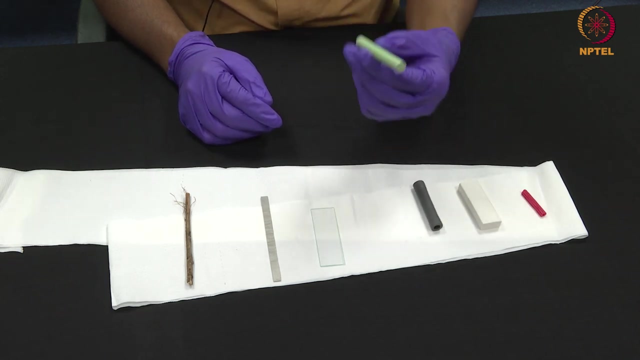 you are seeing in this course. So this display is a different kind of material which all of you might have come across in everyday life. What you see is this is a plastic tube, small kind of tube. This is an eraser, and this is a foam material, a kind of cork, and this is a chalk and this is a glass plate. 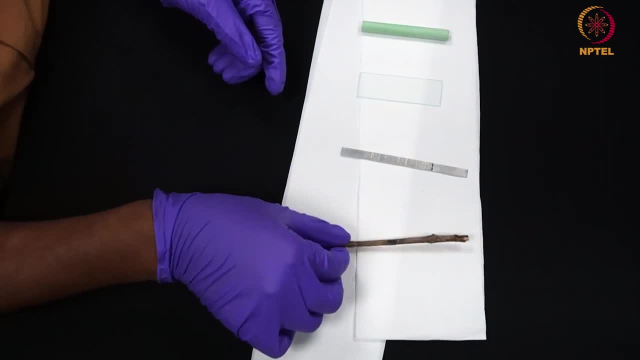 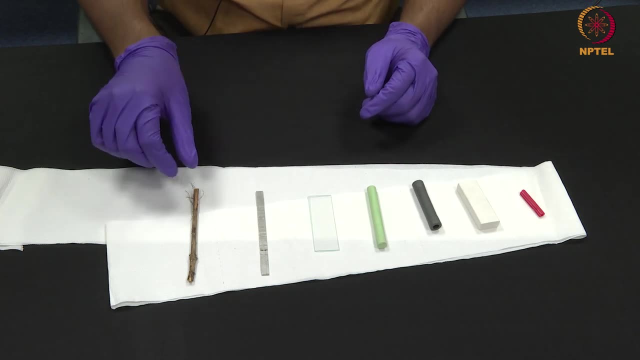 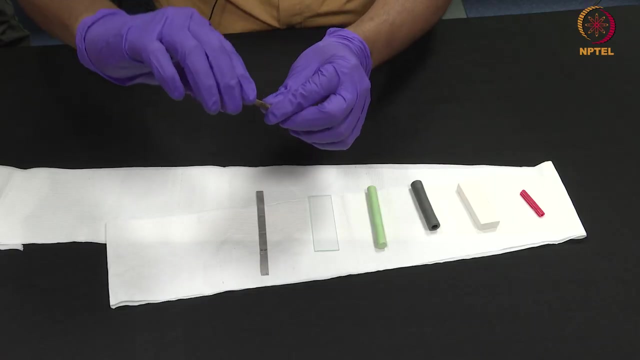 and this is a metal strip and this is a small wooden stick. What I am going to do now is I am just going to take each one of them and trying to apply some force on it. Namely, I will try to do a bending. You just observe what happens: I take this wooden stick and then I bend it. 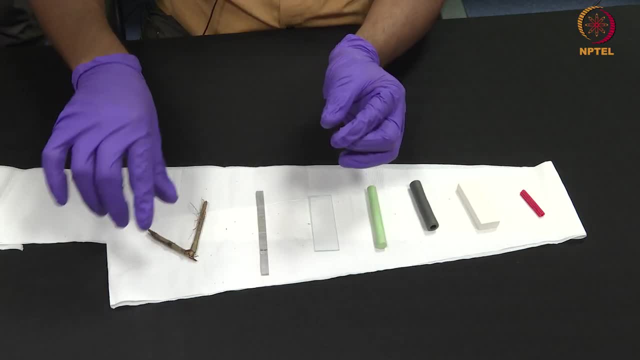 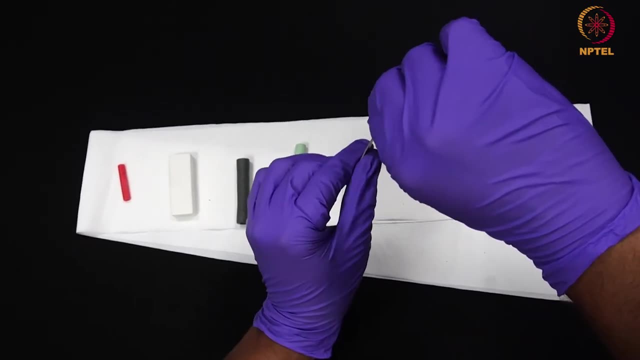 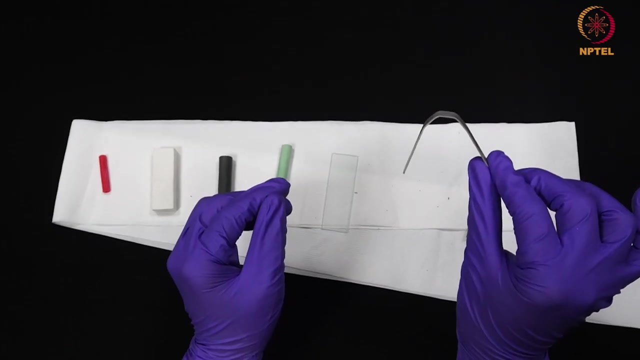 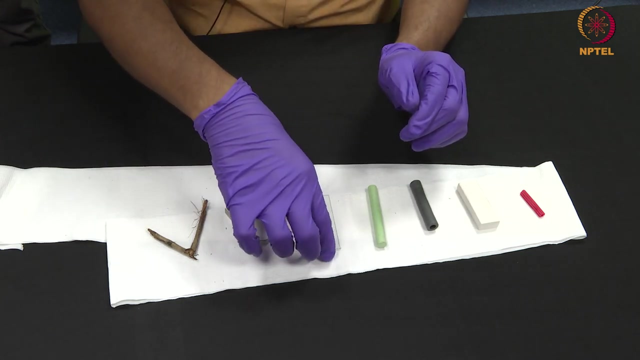 then it breaks like this. Now I will do the same operation on this metal strip. I take this metal strip, I apply a bending force, then it does not break like that, but it is just bending like this and then it stays like that. Nothing happen to that. On the other hand, if I take this a 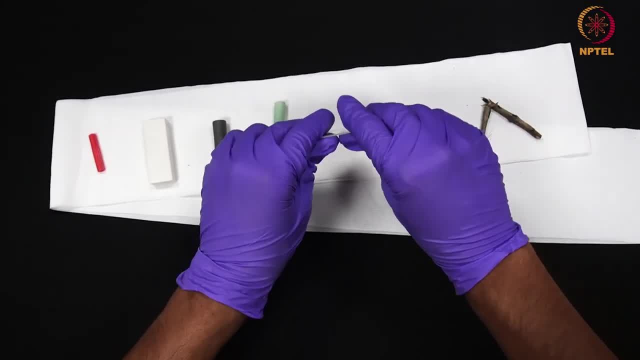 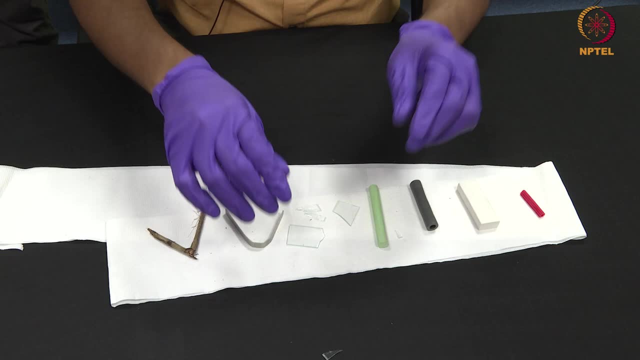 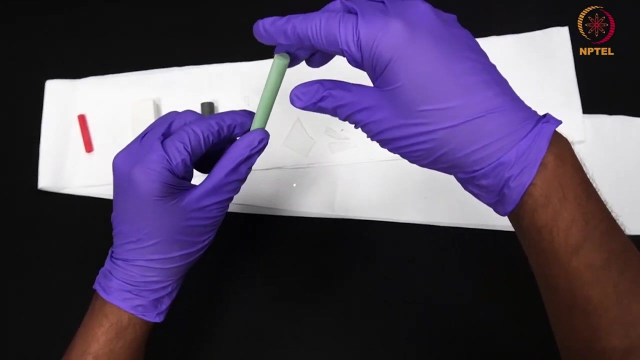 glass strip and then try to bend it. Ok, Ok, it shatters, right. So it is entirely different behavior from the previous material. This is the fourth one. This is a chalk piece. I try to apply this bending force. It just. 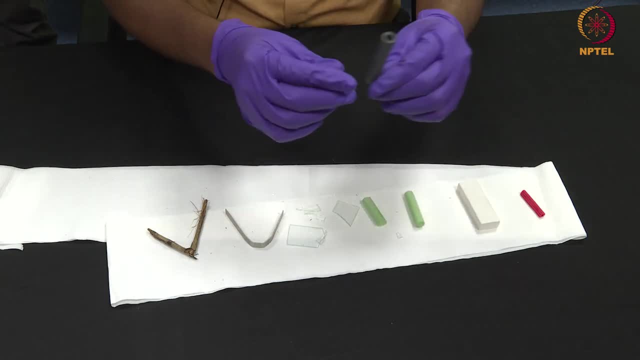 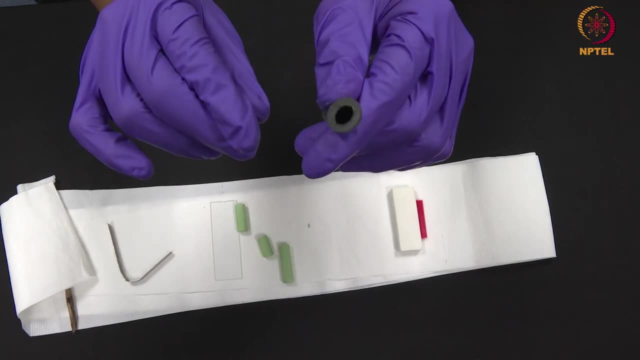 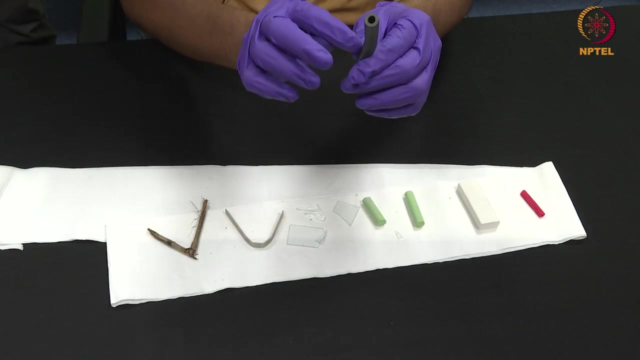 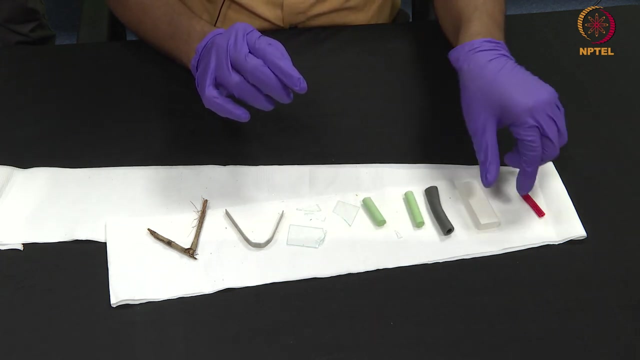 becomes perfectly. two, If I take the cork material and try to do the same bending operation, it bends but it try to come back to its original position, try to recover its position. Still, it retains little bit of that bent in it, right? 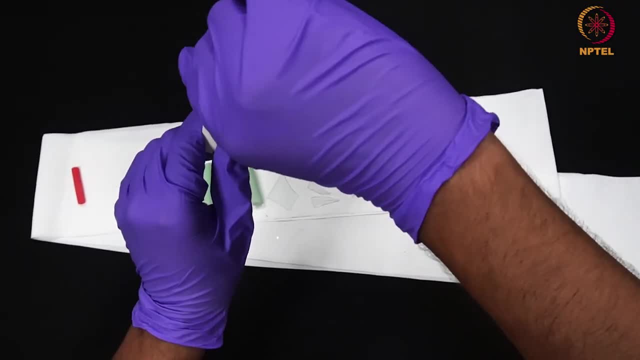 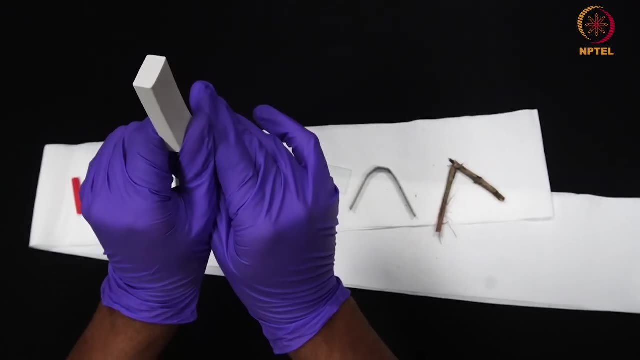 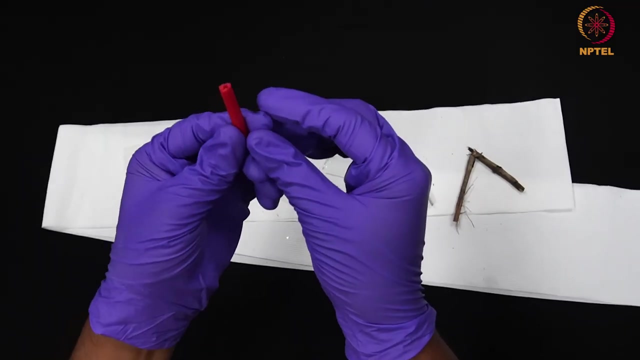 And now this is a rubber. I try to apply the bending force. It bends and it comes back to its original position pretty fast, compared to the previous cork. right Now it is almost become straight. Now the last one. If I take this small stick, if I apply a bending force, it is pretty tough. 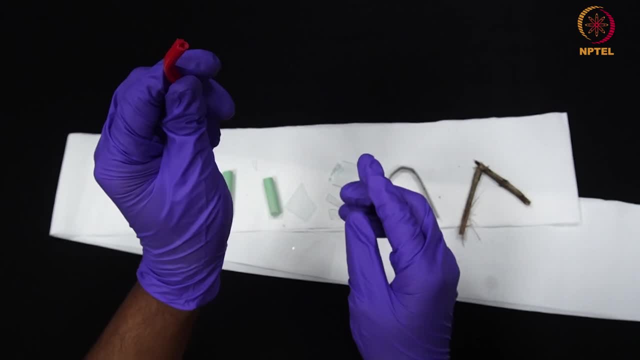 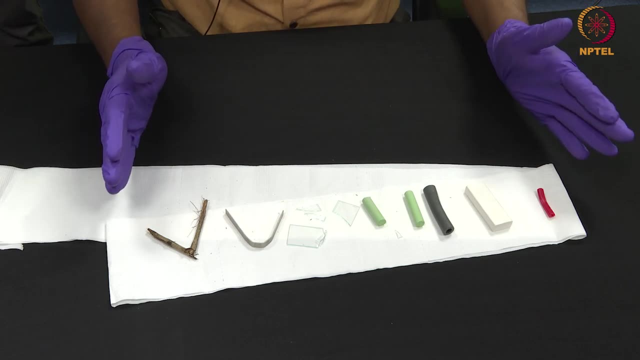 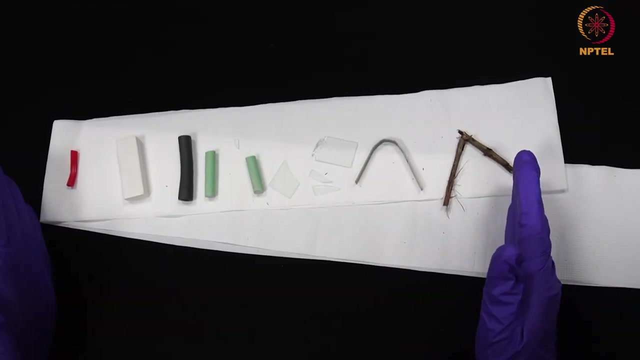 but then it slowly try to come back to its original position. Well, what you now observe from all this? you can actually categorize these materials into a different class of materials. and what you have observed is, even though I applied a similar bending force, 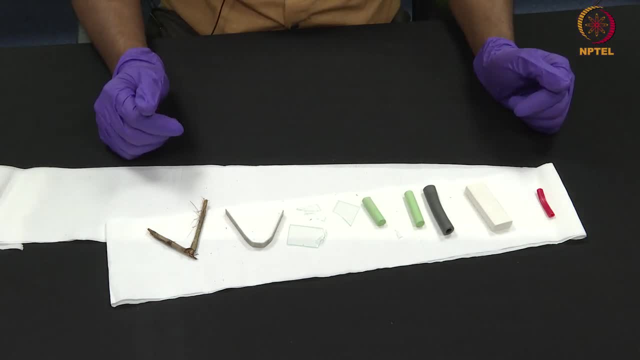 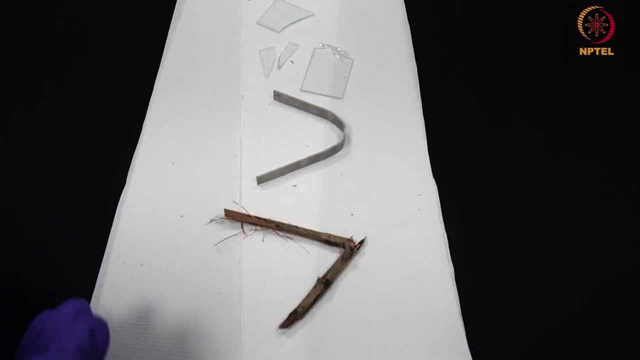 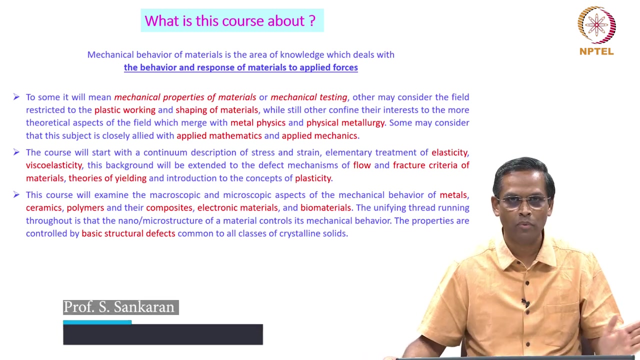 I applied a same force on the same material, Each one responded very differently. right, And this is what we are going to discuss in detail in this course. As you have seen in that video, I have displayed number of materials and its response to the 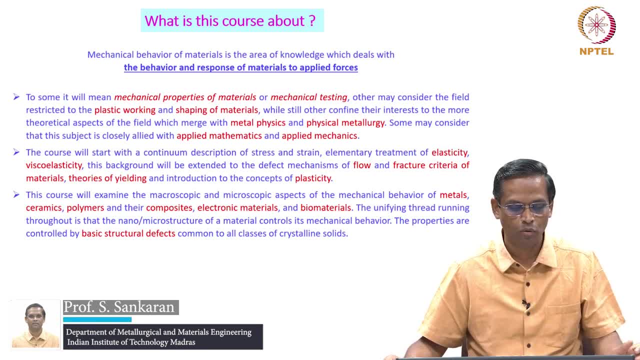 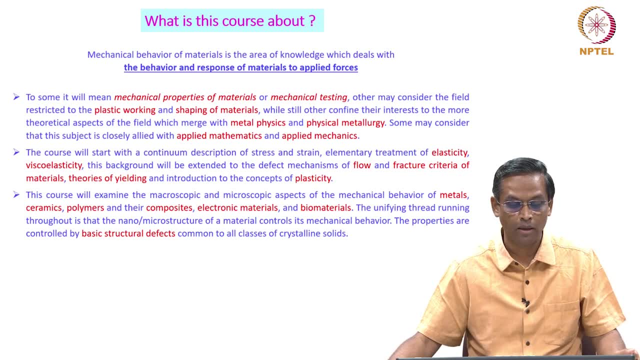 applied forces. So if you look at what is this course, it is mechanical behavior of materials And this is the field of knowledge which deals with the behavior and response of materials to applied forces. To some it will mean mechanical properties of materials or mechanical testing. Other 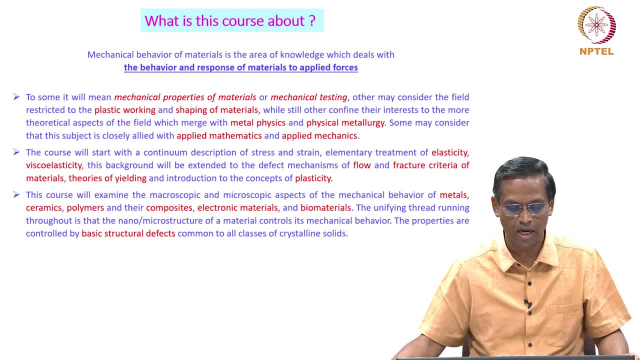 may consider the field restricted to the plastic working and shape of materials, while still other confine their interest to the more theoretical aspects of the field, which merge with metal physics and physical metallurgy. Some may even consider that this subject is closely allied with applied forces. 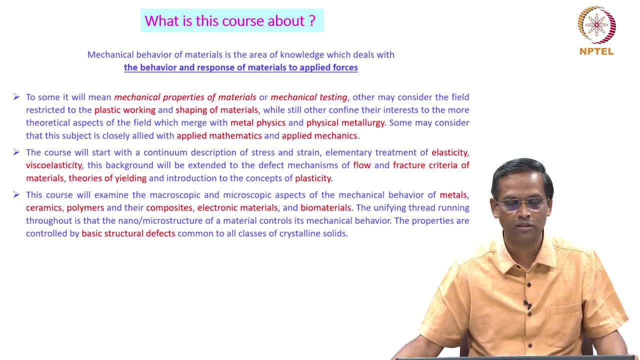 So this is the field of knowledge And this is the field of mechanical testing. Some may even consider that this subject is closely aligned with applied forces, So it is extremely related to natural too. in nature, It is going to cover a lot of subjects together under one umbrella. 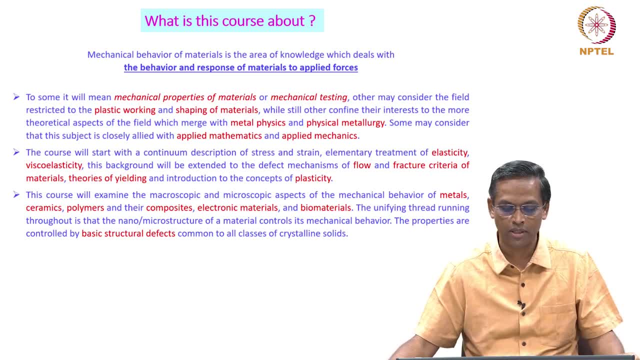 Hence the course will start with a continuum description of stress and strain, elementary treatment of elasticity, viscoelasticity, And this background will be extented to the defect, mechanisms of flow and fracture, criteria of materials, theories of yielding and introduction to the concept of plasticity. 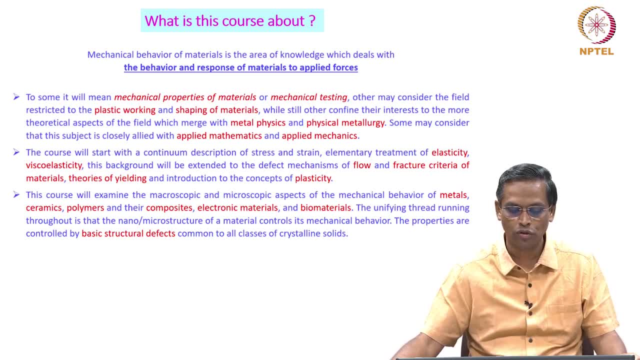 The course will examine the macroscopic and microscopic aspects of the mechanical behavior of metals, ceramics, polymers and their composites, electronic materials and biomaterials. The unifying thread running throughout is that the nanostructure or microstructure of a material controls its mechanical behavior. 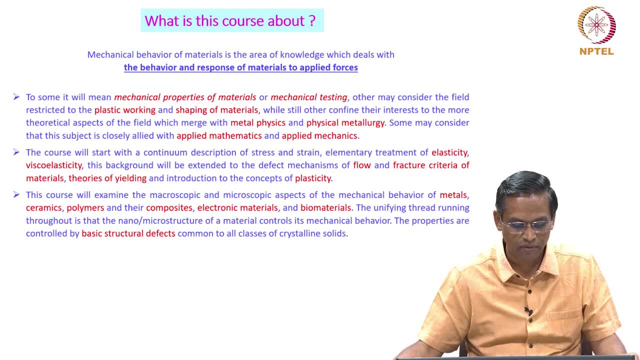 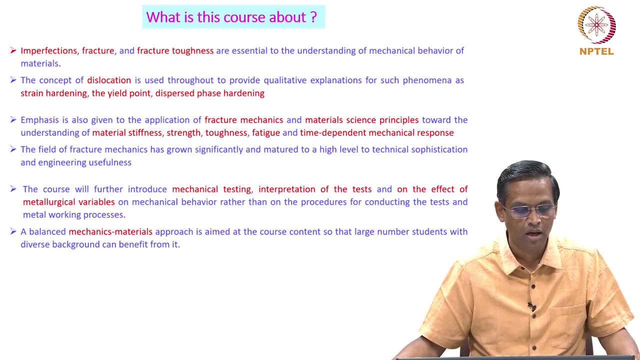 The properties are controlled by basic structural defects common to all classes of crystalline solids. Imperfections, fracture and fracture toughness are all essential to the understanding of mechanical behavior of materials. The concept of dislocation is used throughout this course to provide a qualitative explanation. 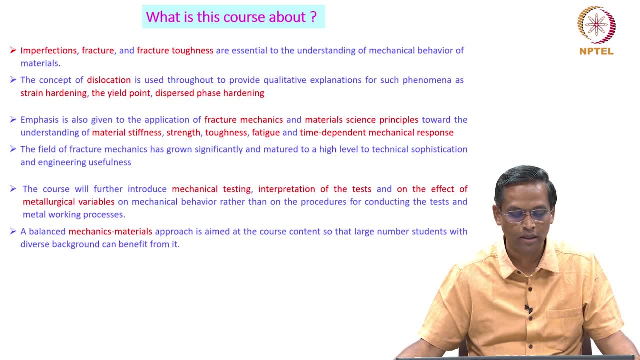 for such a phenomenon as strain hardening, the yield point dispersed phase hardening. Emphasis is also given to the application of fracture mechanics and material science principles toward the understanding of material stiffness, strength, toughness, fatigue and time-dependent mechanical response. 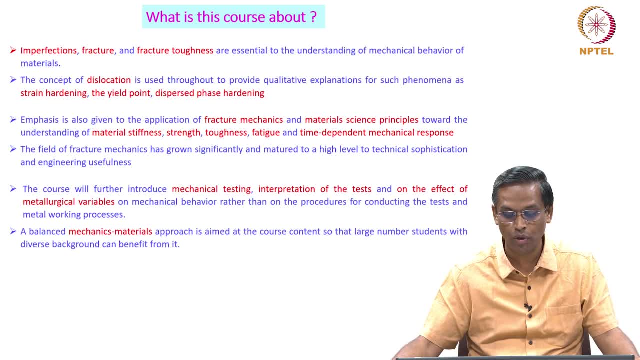 The field of fracture mechanics has grown significantly and matured to a level to technical sophistication and engineering usefulness. The course will further introduce mechanical testing, interpretation of tests and on the effect of metallurgical variables on mechanical behavior, rather than on the procedures for conducting the tests and metalworking processes. 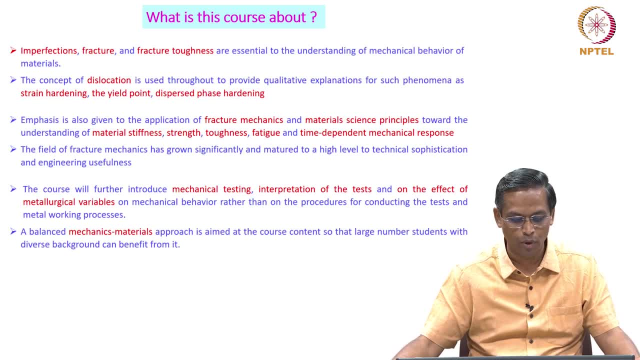 So a balanced mechanics materials approach is aimed at the course content so that large number of students with diverse background can be involved in the course. The course will also introduce a series of technical and mechanical testing and interpretation of the materials. The course will also introduce a series of technical and mechanical testing and interpretation. 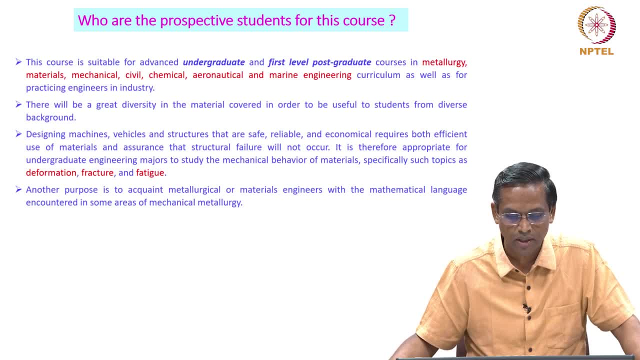 of the materials. The course will also introduce a series of technical and mechanical testing and interpretation of the materials. So who are all the prospective students for this course? As I just mentioned in the beginning, the course is suitable for advanced undergraduate and first-level postgraduate courses in metallurgy materials, mechanical, civil, chemical, aeronautical. 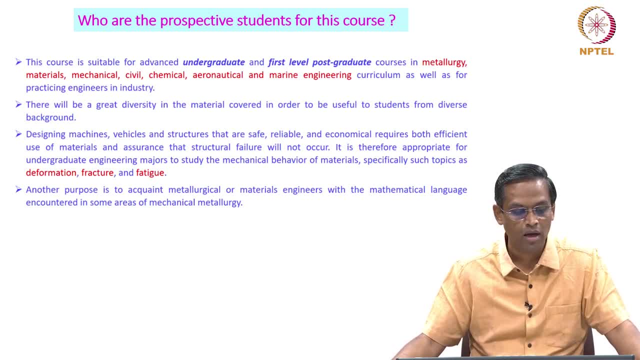 and marine engineering curriculum, as well as for practicing engineers in the industry. There will be a great diversity in the material covered in order to be useful to students from diverse backgrounds. diverse background: Designing machines, vehicles and structures that are safe, reliable and. 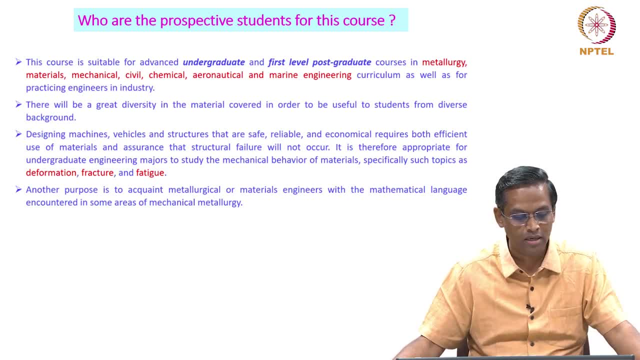 economical requires both efficient use of materials and assurance that structural failure will not occur. It is therefore appropriate for undergraduate engineering majors to study the mechanical behavior of materials, specifically such topics as deformation, fracture and fatigue, and so on. Another purpose is to acquaint metallurgical and materials engineers with